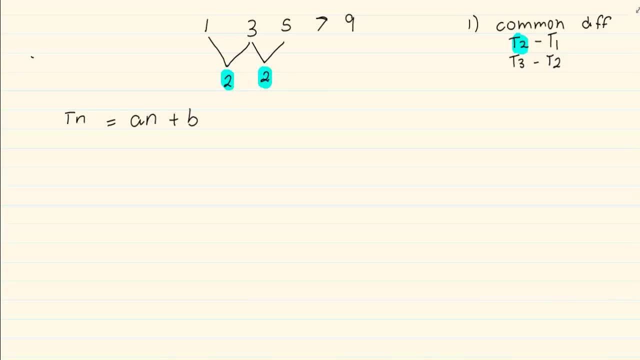 at the step. So for now we have: tn is equal to 2n. How do we solve for b? If you were counting in multiples of a? So if I was counting in multiples of a, So in this case a is 2.. So I'm counting in multiples of 2.. 2,, 4,, 6, 8.. 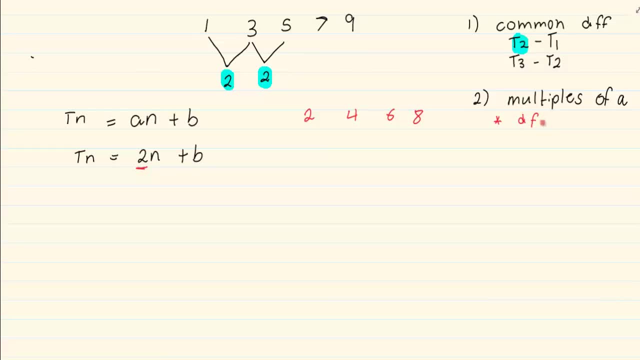 Now what I'm trying to do is: what is the difference between tn and a? So tn is equal to 2.. So tn is equal to 2.. So tn is equal to 2.. Now I have to write the difference between the multiple. 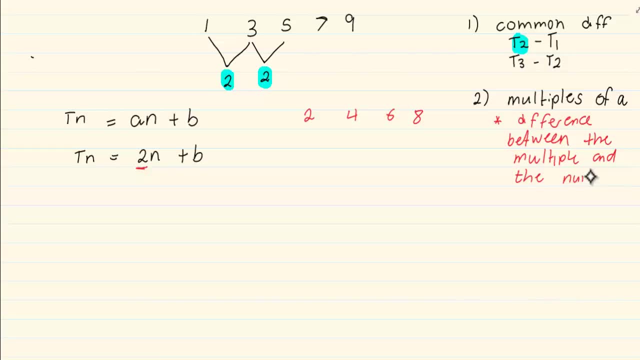 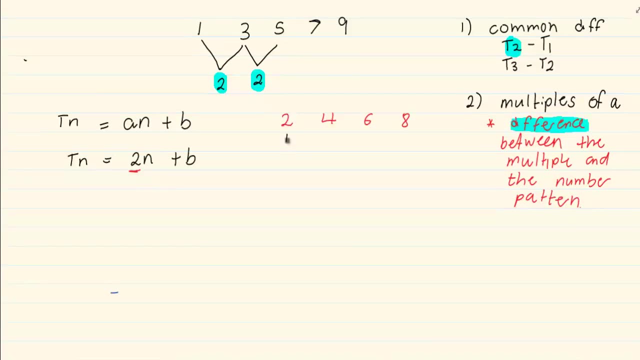 and the number pattern. Underneath I am going to write the number pattern 1,, 3,, 5,, 7.. Now, Now, what we're looking for is: what is the difference between the multiples and the number patterns? What is the difference between the multiple and the number patterns? 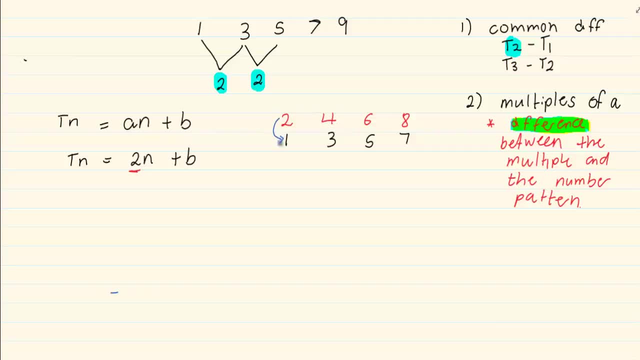 So to move from 2 to 1,, what do I have to do? To move from 4 to 3, what do I have to do? You would notice that I would have to subject 1.. So my formula becomes: Tn is equal to 2n minus 1.. 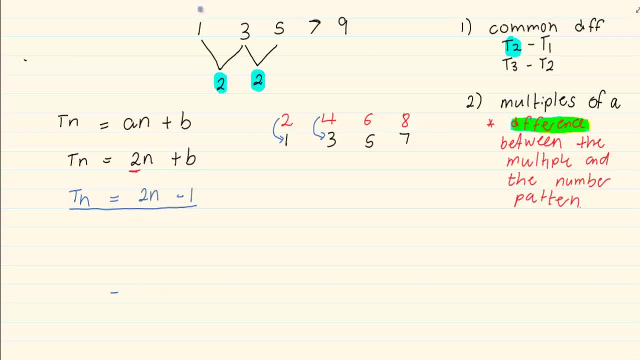 Now let us check this. In our previous video, we discussed that this is T1,, meaning n is equal to 1.. So if I had to substitute n as 1,, I should get the answer 1,, which is exactly. 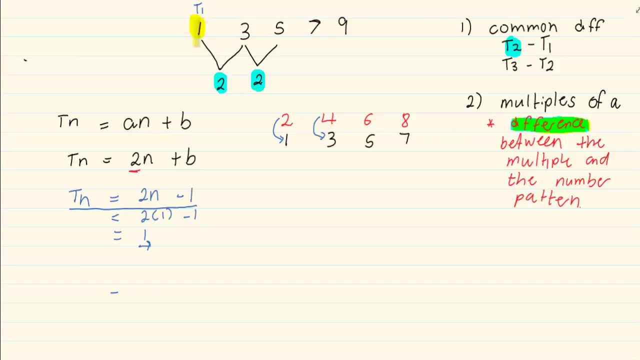 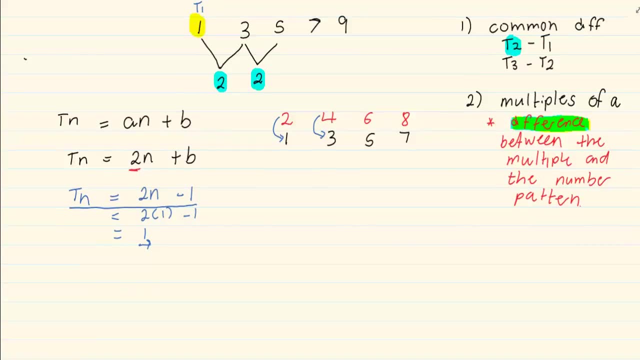 what the number pattern states. Now let us try another one working with a negative. Okay, if I am given the following number pattern: 10, 7,, 4, 1.. Now the first step is we're going to check what is the common difference.